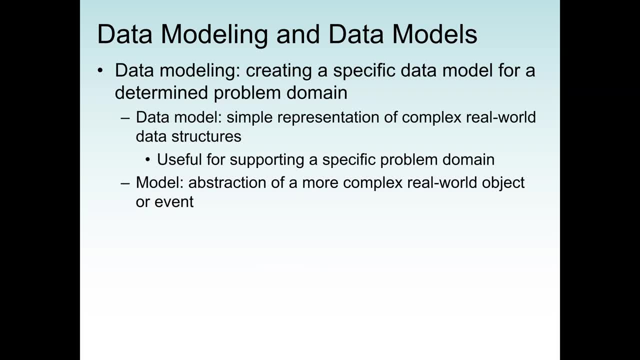 again, redo it or to correct the mistakes. And when we create a data model, anytime we can communicate with other professionals in the field and we can again modify it, And it won't cost much time or financial. So data model is very important in almost every. 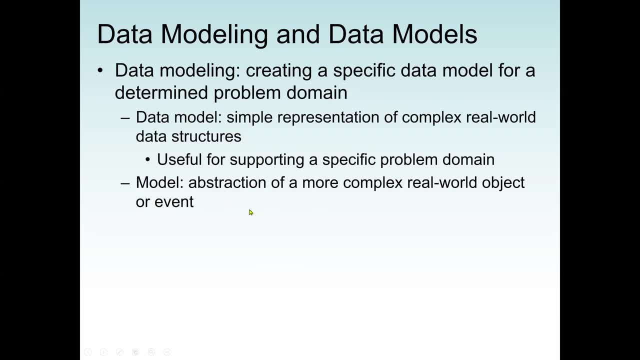 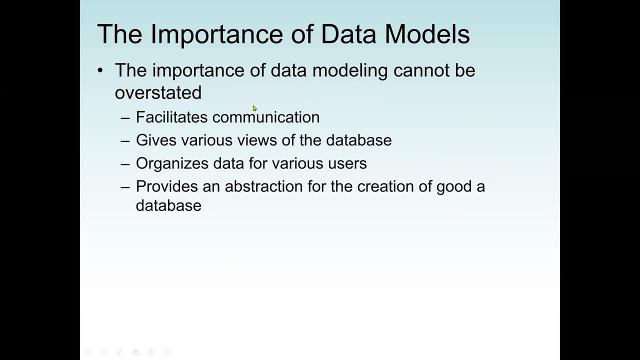 manufacturing industry. So a model can be an abstraction of a more complex real world object or event. So the importance of data model: as we said, it also facilitates communication. So if we create a model, we can communicate with our project sponsors or the stakeholders in the 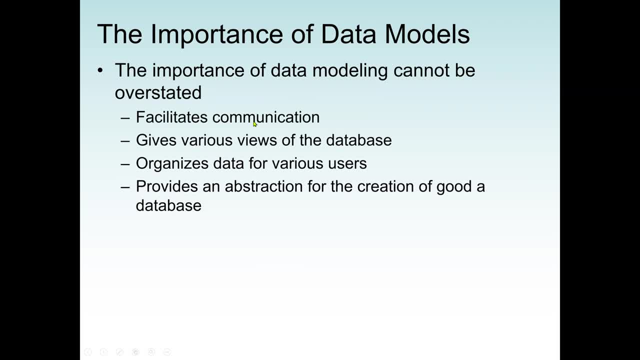 project how they want the system to be, And modifying a model is more quicker and less costly than developing the system. In some other techniques we can, instead of developing the real system, we can create a prototype. So that's another software engineering technique where by- instead of- 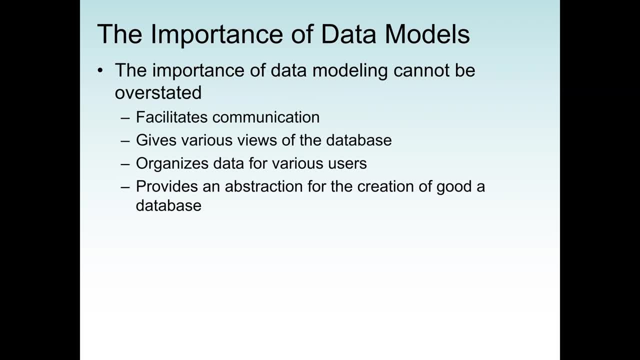 developing the real system, we can create a prototype. So that's another software engineering technique where by, instead of creating a model, we create a prototype of the real system, And that also works. So the importance of data model cannot be overstated. It facilitates communication. It also gives various views of the database, Also organizes data for 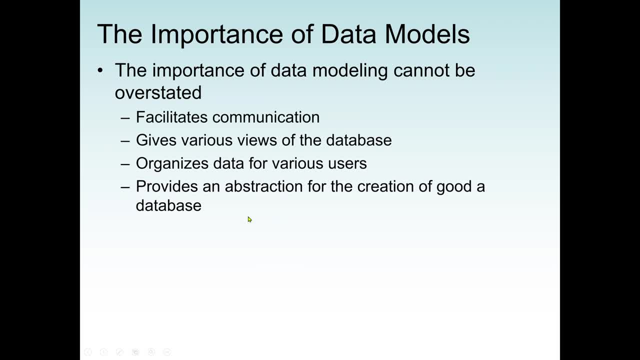 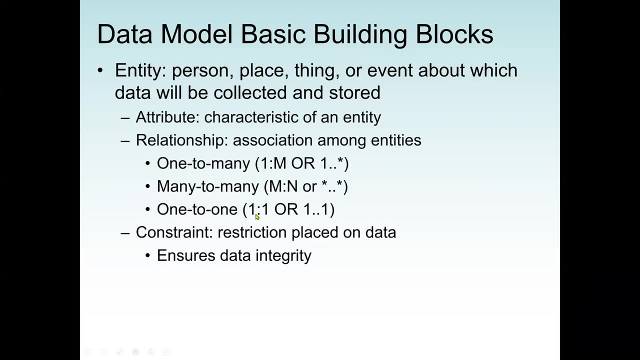 various users and also provides an abstraction for the creation of a good database. So again, this course is a database management system. So when we talk about data model, we are talking about again designing a data model for a database application. So normally in a data model, basic building blocks: 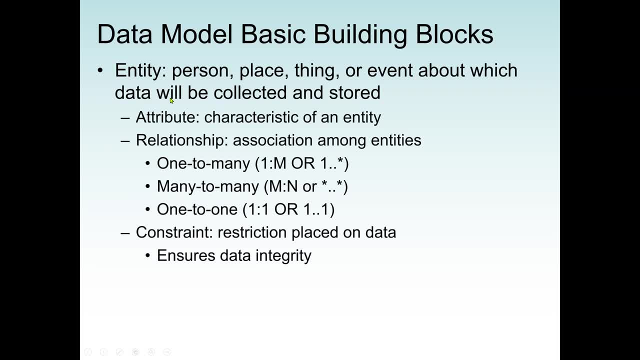 in database management system. number one would be an entity. So an entity can be a person, place, thing or event about which a data will be collected and installed. So, for example, if I want to design a database for, let's say, a bank or financial institution, maybe one of the entity I would consider would be 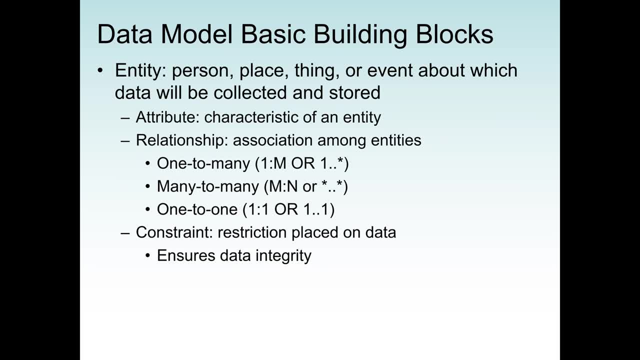 customers And also I have to know the characteristics of the customers, which would be customer last name, address, place, etc. These are the data I want to store about a customer. So a customer is an entity And also an attribute. So we talk about the attribute- Attribute to be the characteristics of an 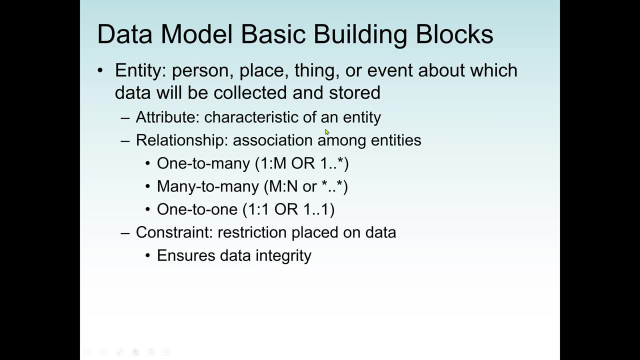 entity. So if it's a student, I want to store data about a student. A student is an entity: Student, grade, last name, address, major, etc. That would be the characteristics of an entity. Then we also have a relationship. A relationship would be the association among entities. So, for example, in a 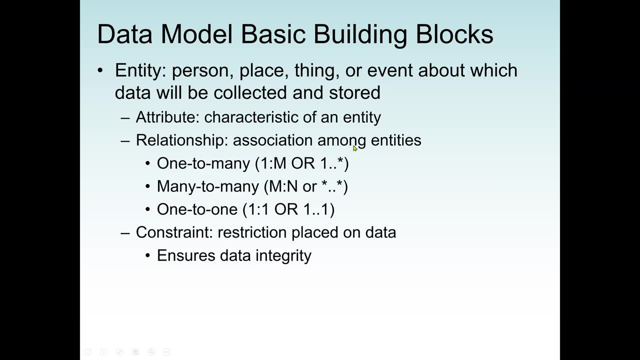 student. I may have a student entity and the characteristics of the entity of student can be name, first name, address, grade and also I may have another entity called a course, the cost. I have a course ID, course name, number of credit for the course. this would be the course entity. now I can create a relationship between two. 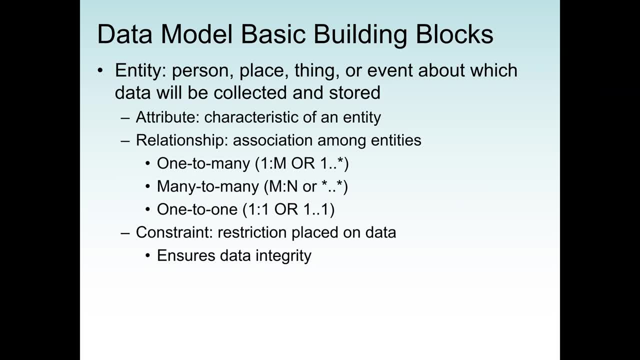 entities, or more. this relationship is what we call the association among entities. can be three different times. we can be one to many, many to many, one to one. so, for example, based on the business rule of the of an institution, a university, we can say that, okay, one student can take only one class at a. 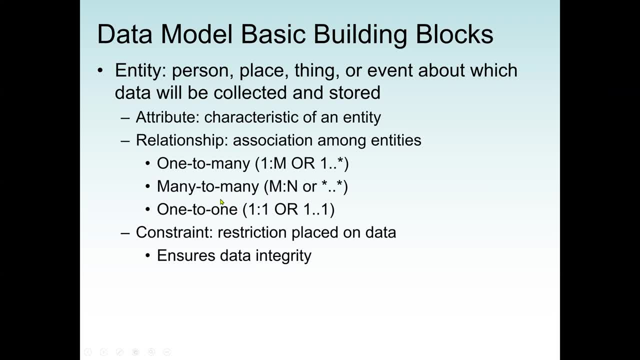 time, because the semester runs for only five weeks. or we may say that one student can take two or one or two classes- you got a semester runs for eight weeks. or a student can take four up to four classes, because the semester run for sixteen weeks. so these are the business rules. so normally association and the 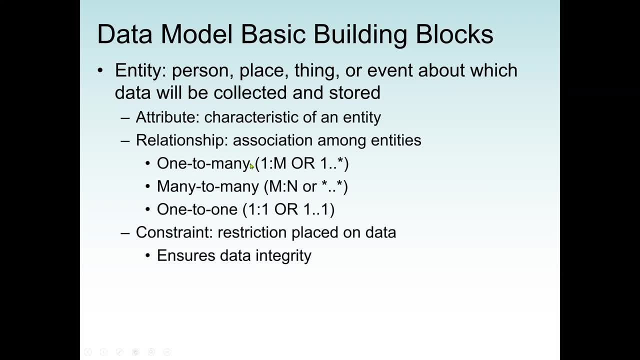 type of relationship we may have between two entities. we normally going to generate a type based on a business rule of the organization. so in database management system we have three different types of relationship, as we said earlier: one to many, many to many and one to one. example: one student can take only one class at a. 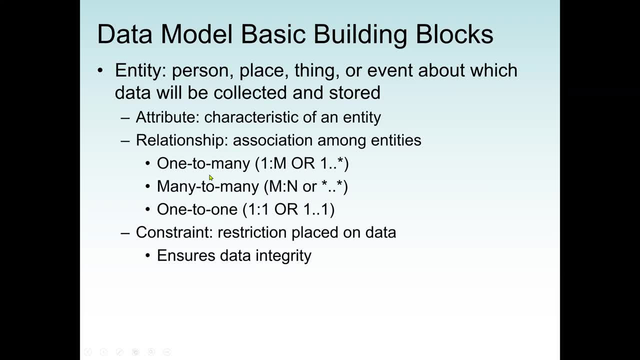 time one student can take one or many classes, or many student and take many classes. then we have what we call the constrait. the constrait will be the restriction which would be placed on the data. it also ensured the data integrity. then we may discuss it by this when we start data modeling. to go on, 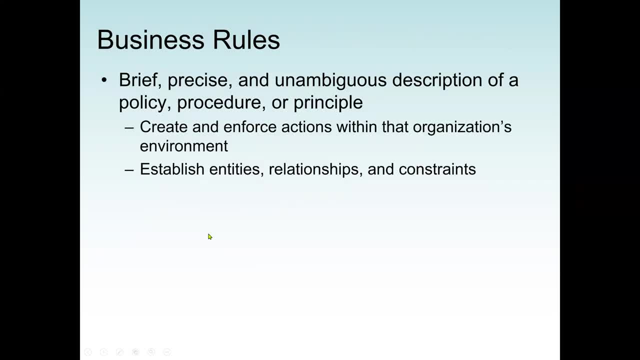 next slide topic. so business, through the most important process of data model or designing a database, because most of the relationship we are going to play between entities will be generated from the business room. so a business who can be the brave, precise and also ambiguous description of a policy procedural. 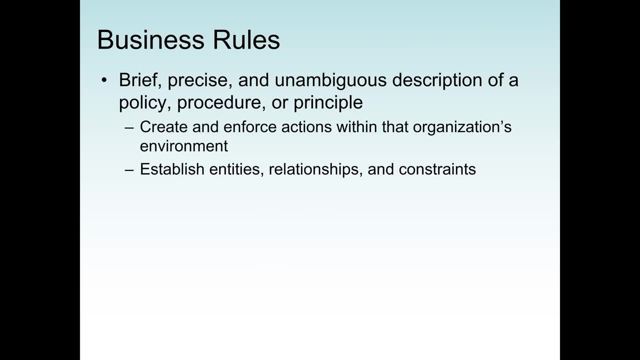 principles. we have a university. the university policy said one select article, one class at a time, while we have a parking institution we said that many customers can open one or many accounts. so we create and also enforced actions within that organization environment. business really get, create and also force actions within the organization. 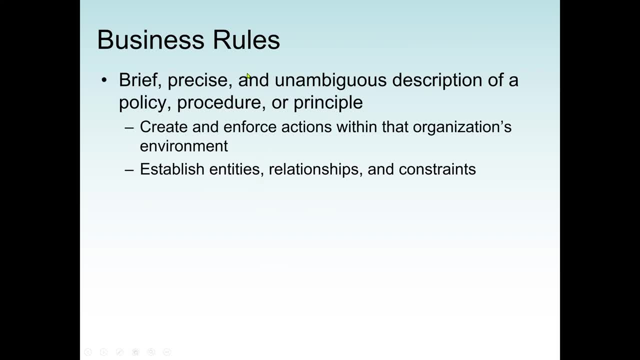 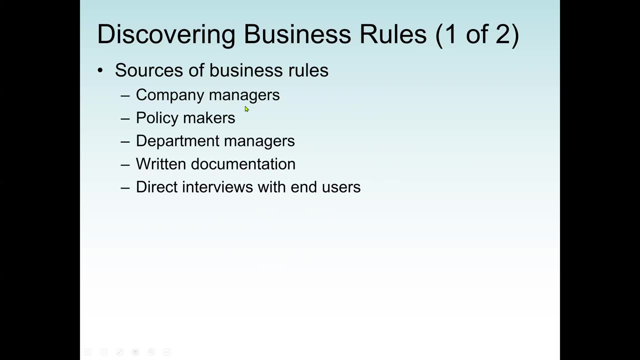 business room again create and also forced actions within the organization. Also, as we said, the business rules will establish entity relationships and constraints. So how do we discover business rules? The source of business rules can be the company's managers. they may come up with the policy. 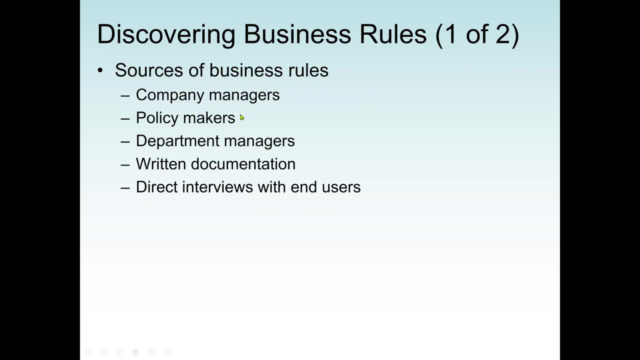 of the organization or policy makers or department managers. they may come up with their own standard procedure of doing business or written documentation. also direct interview with end users, based on how the end users use the system when they come up or how. 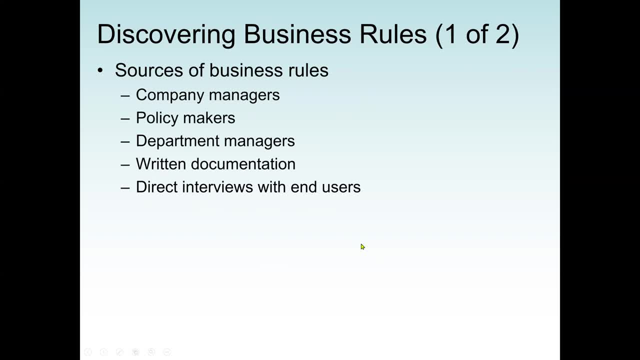 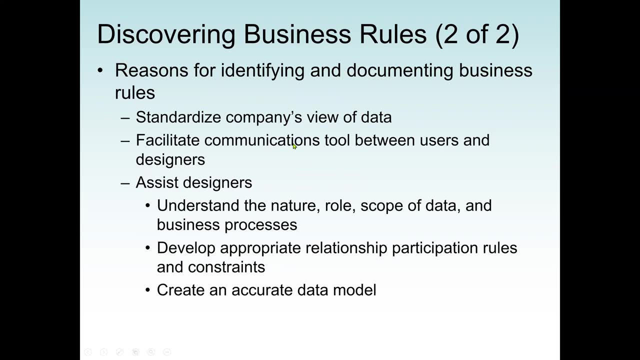 they do their business operation when they come up with the business rules. So reasons for identifying and documenting business rules: One is to standardize the company's view of data. Standardize Then also to be able to facilitate communications too, between the users and designers. 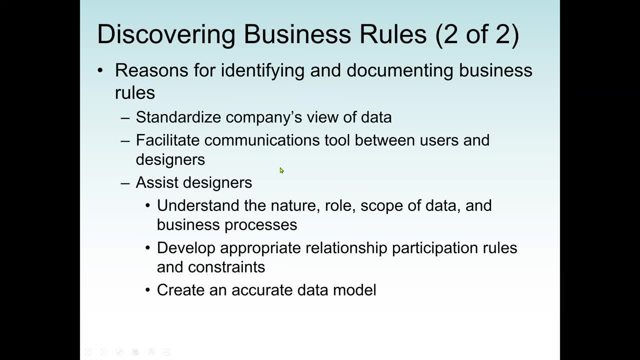 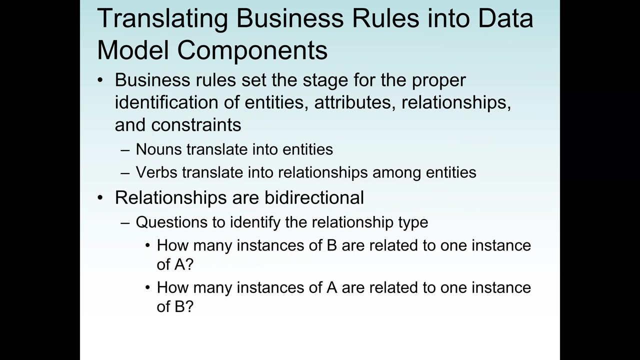 As we said earlier, the business rules are the core way of getting the type of entity relationships. Also assist designers to understand the nature, the role, the scope of data and business process. develop appropriate rules. Create an accurate data model. Business rules normally set the stage for the proper identification of entities. attributes: 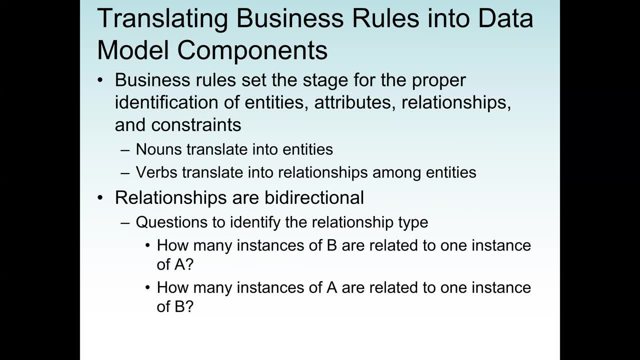 relationships and constraints. And also when we are designing our database system, always we use the nouns to represent the entity, Such as the student employee or the customer, And finally the baseline. Then the verbs we translate into actions among a relationship, among entities such as student. 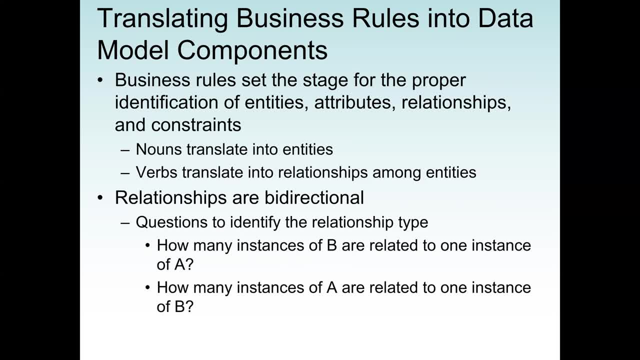 can take one class. take: or employee manages one department, or employee works in one department, or one or many departments, or we can say employee assigned to one or more departments. So we can see that the relationships will be verbs and the entities always are nouns. 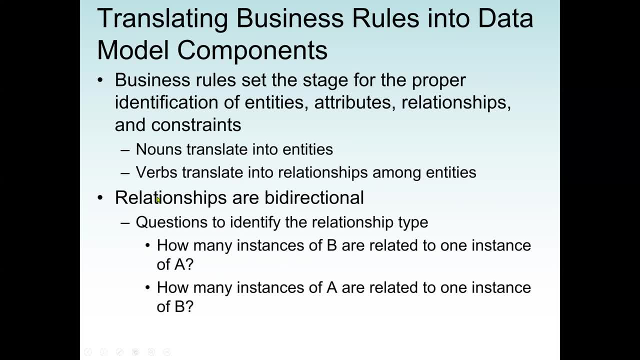 Also, relationship can be a bi-directional. So we say one student take one class. we can say one class can be taken by one student. So how many instances of B are related to one instance of A, or how many instances of A are related to the other? 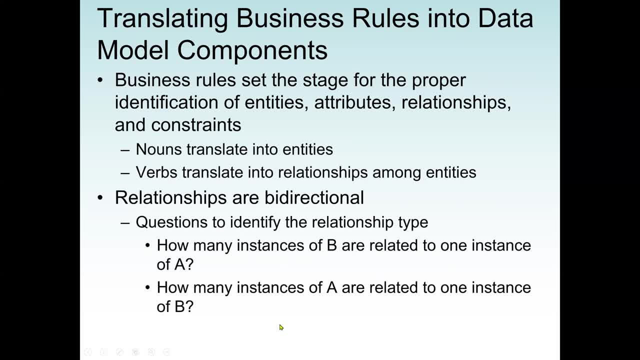 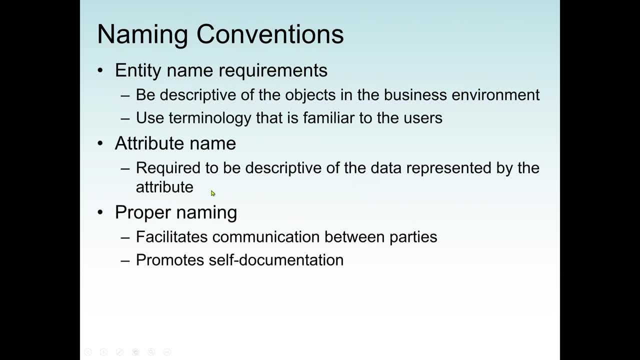 So relationship again can be bi-directional. Then also the naming conventions is very important in the design process of a database system, management system. So entity name requirement, this is just a conventional name, it's not a rule. So here we say be descriptive of the object in the business environment. 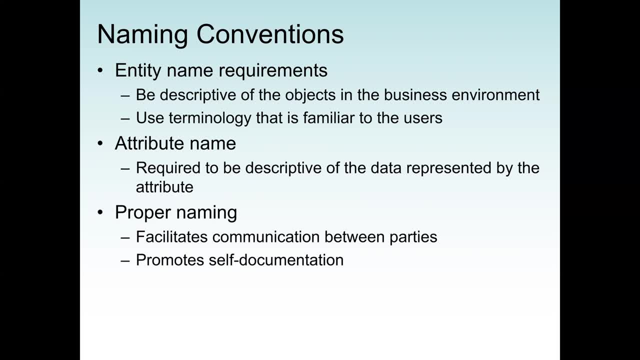 For example, if I have an attribute last name or last name, Okay, So I want to store last name. I don't want to name the attribute X or Y, right? I will name it last name so that we know the content of it. 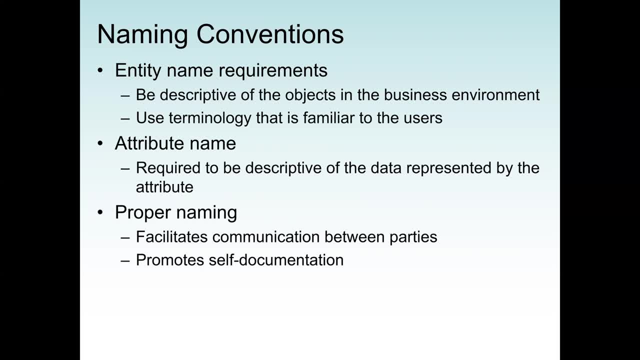 Same thing: a table, a table entity that I want to. I want to store a data by an entity. I will name that entity by that very type, So I may have a student table- I'm not going to say market table- and in the market table. 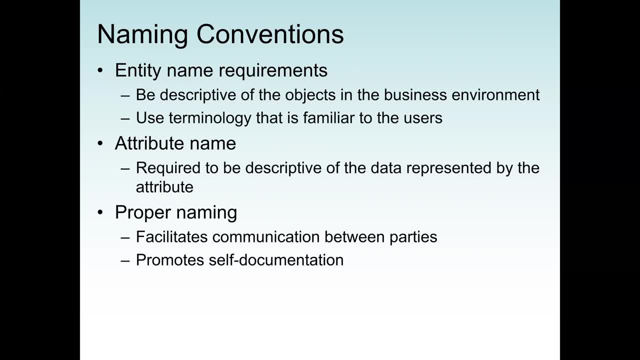 I'm going to store- Okay, I'm going to store student information. So naming convention always have to be related to the type of information you are storing, either in the entity or the attributes. also, So we say, be descriptive of the objects in the business environment. 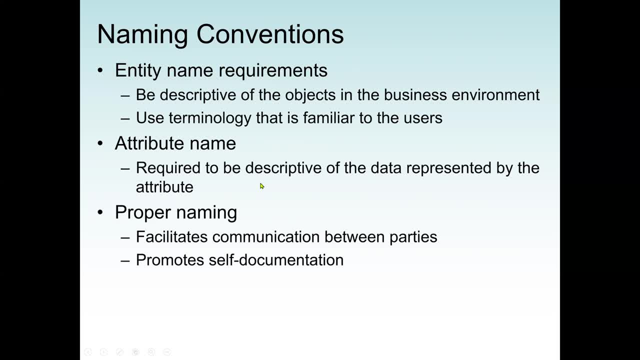 Use terminology that is familiar to the users. Also, attribute name required to be descriptive of the data represented by the attributes. So last name, address: city. If I want to store the city Name of the entity, let's say student or employee, I will name the first city. 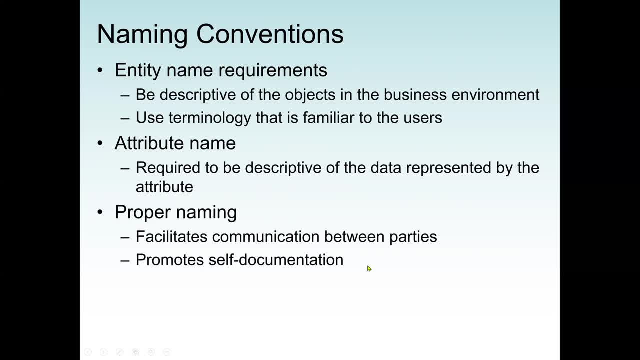 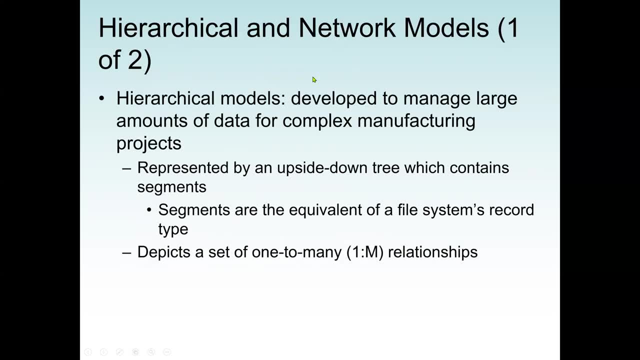 Also proper name. we should facilitate communication between parties, promote self documentation. Now we have different types of modeling. Here we discuss about hierarchy and also network models. So the hierarchy models normally develop to manage a large amount of data, For example for complex modeling for trial projects. 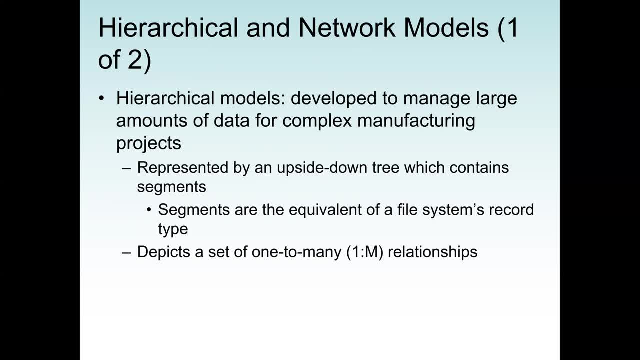 So that's why it's in hierarchy form, So it's kind of we're going to decompose it from top down And this is can be represented by upside down tree which contains segments. So segments are equivalent of a file system record type. 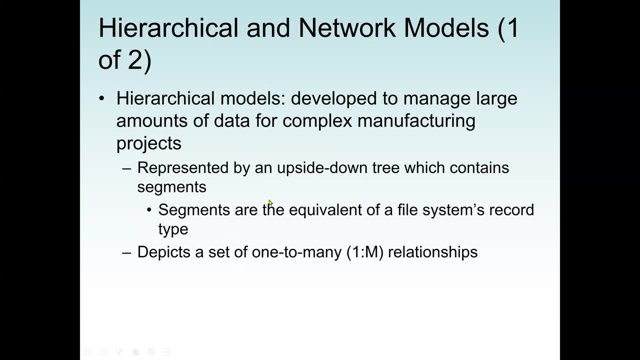 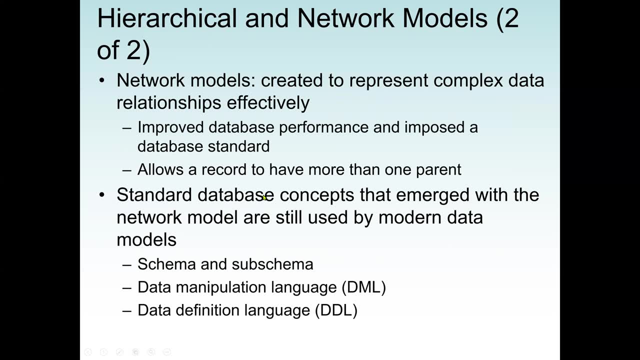 And we can show it to a set of one to many relationships By network model, normally created to represent complex data relationships Effectively. Here it's going to improve the database performance and impose the database standards. Also, it will allow a record to have more than one parent. 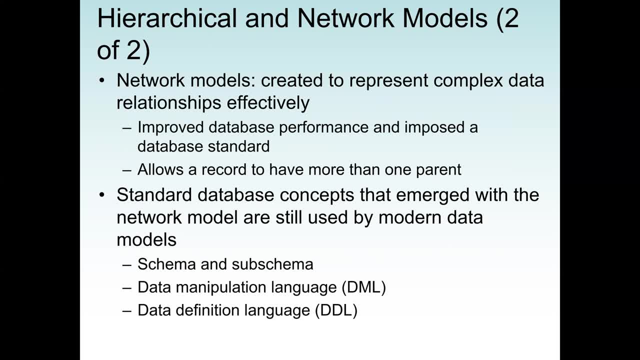 The standard database concept that emerged with the network model, which are still used by modeling data models can be a schema, soft schema, data manipulation language, data definition language, Data manipulation language and data definition language. So data manipulation language and data definition language. 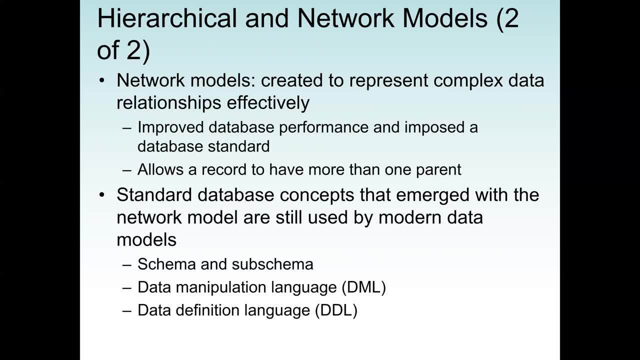 So data manipulation language and data definition language. Data definition language is a two major part of sequential query language. So data manipulation language is when you want to write a query like select statements. I want all the students that got a grade of A, So I'm going to write a query. 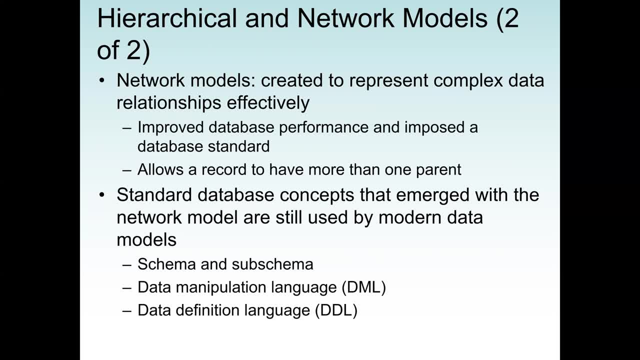 A query is part of the data manipulation language. Data definition language. example of the script can be create or delete, So data definition language. Normally, The idea is to create a database that uses internal logical information. So we're using it To create a database that uses internal logical information. 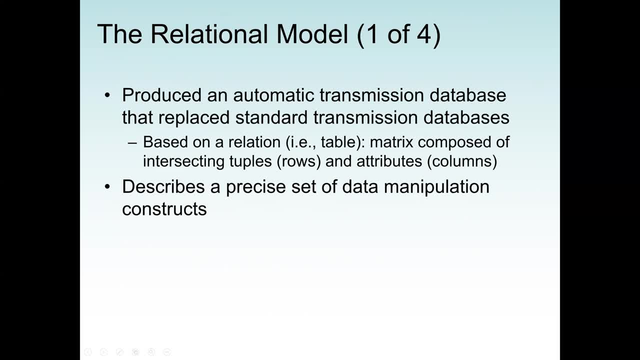 So a relationship model normally produce an automatic transmission database that replace standard transmission databases. So relational model normally is based on relational relation, Relational table. so when we say relational database system we mean that we need a database that normally is based on table system. a table normally consists of rows and columns. there will also be the records of 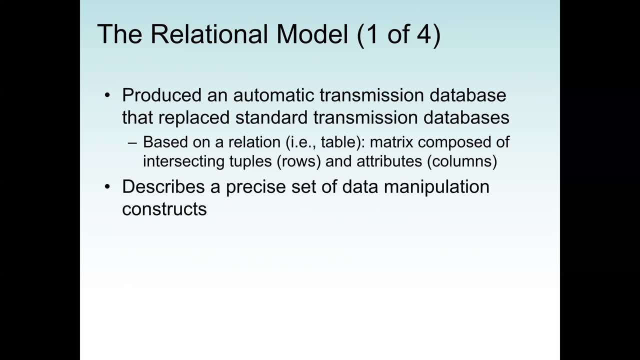 one person or one entity and the columns will be the fields which are: the column is the scalar unit, then the smallest unit it will be the characteristics of the entity. so we say the table is almost same as matrix rows and column. so we see a matrix composed of intersecting. 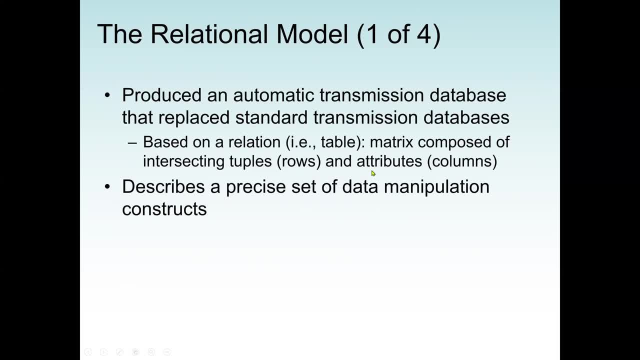 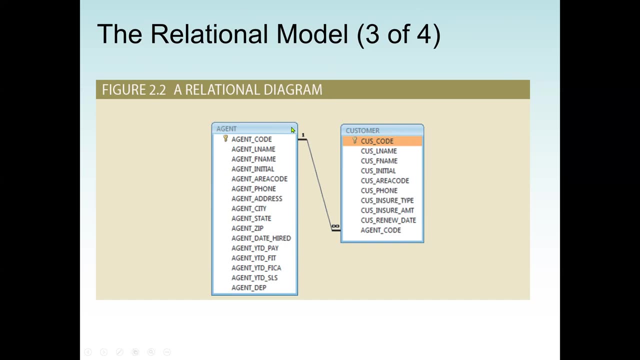 tuples, which is the rows, and also the attribute, which is the column, and also describes a precise of data manipulation constructs. so this is an example of a relational model. we have two. this is created using the microsoft assets, so we have the agent database or we say, in this case, a relation or a table. this is a database system consists of two. 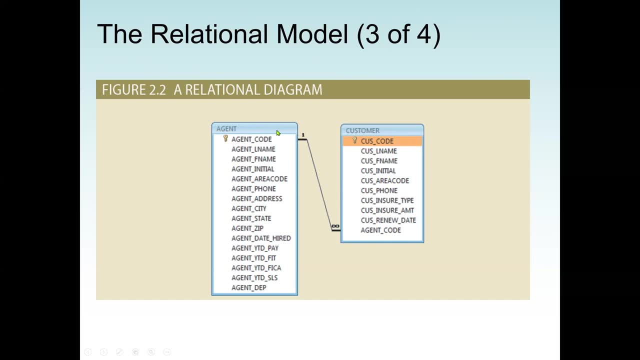 tables, an agent table or relation and a customer and we can see the relationship here. one customer applied- sorry, one agent maybe can represent one or many customers and our primary key fit for agent is agent code and we can use that. we are using the agent code in the customer. 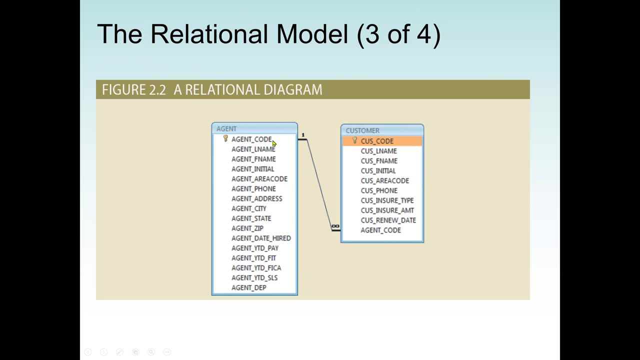 relation. so agent code is called the primary key field in agent, then agent code in another table- in this case customer will be called a foreign key. so a foreign key is a key that is a primary key field in another table. and the main reason of foreign key is to allow us to create a relationship between the two tables. so when i'm creating this, 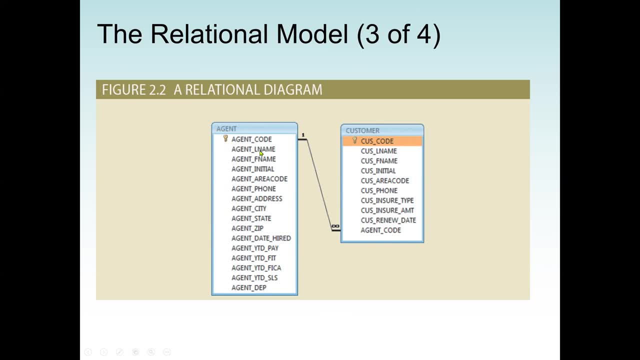 between these two tables, agent and customer. i'm using the field name agent code and also agent code in the customer to create the relation. so you can see that in agent code as a primary key field we cannot have the same primary key field twice because primary key field, as we said. 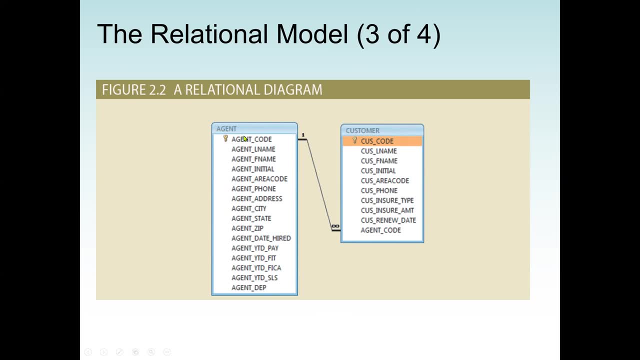 is uniquely identified each record, so the entry must be unique. for example, we don't have no two elements on the same table, but we do have a no two set of units. so that means that which is one table means an agent code. so that means that the agents creates information about the. 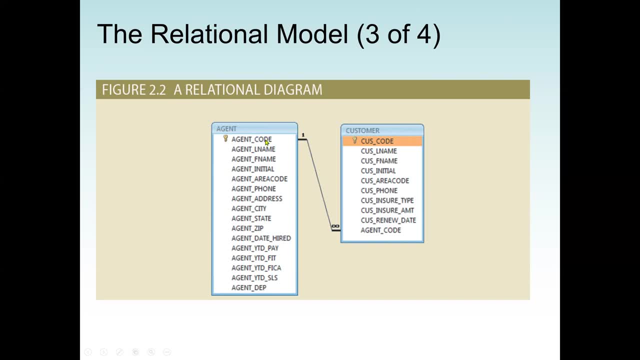 time frame and code 1, 1, 10 times representing each customer, because this is a foreign key. but in an agent table, agent code is a primary key field. we can have the same code to us, but if it's a foreign key or something we use the 10 second way key. 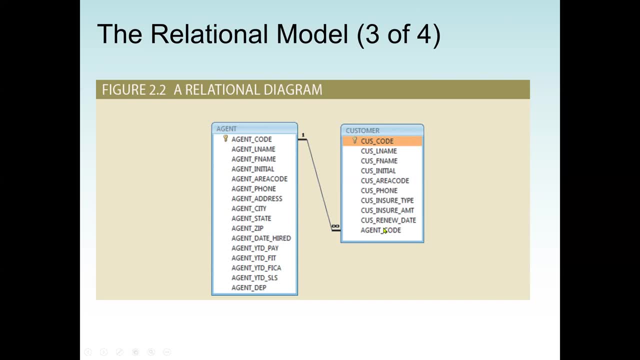 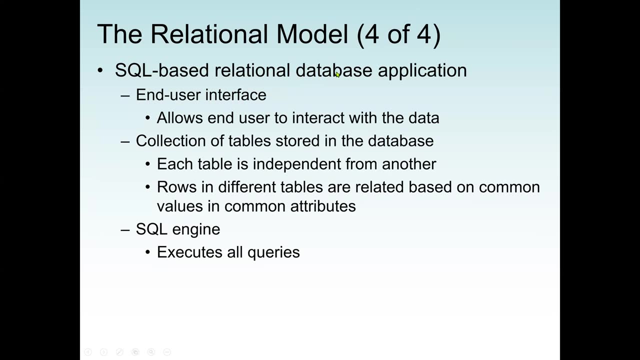 we can have as many same field, as many as we want. so SQL based relational database application we mentioned earlier. SQL stand for sequential query language and sometimes we call it structure query language, and it consists of major two parts, that's the data manipulation part and data definition. 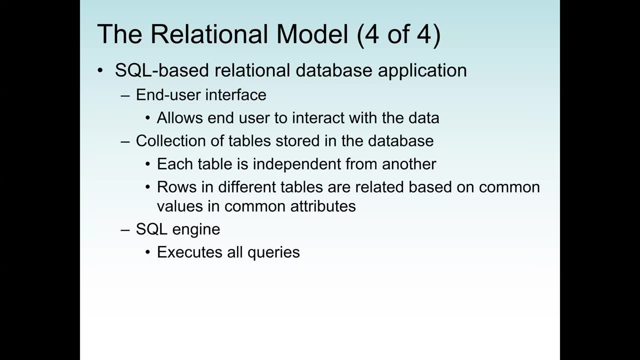 part or so it's a man precious for the select queries and data manipulation part. part is to create or develop you entities relationship etc. so the end-user interface allowed a user to interact with the data when the collection of data table store in a database. each table is independent from another. roles in different tables are: 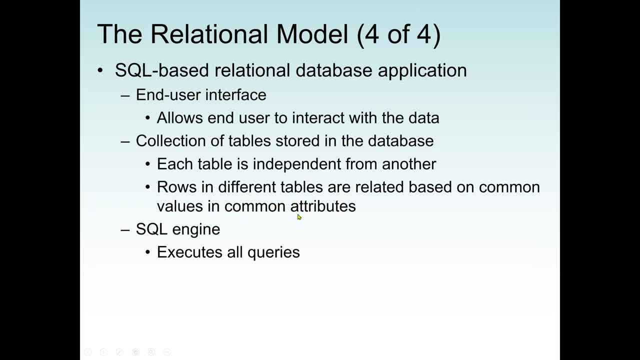 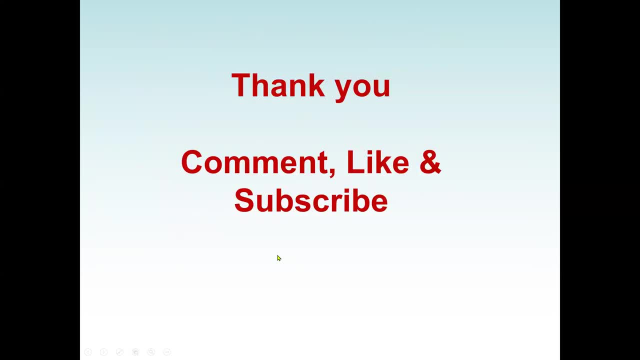 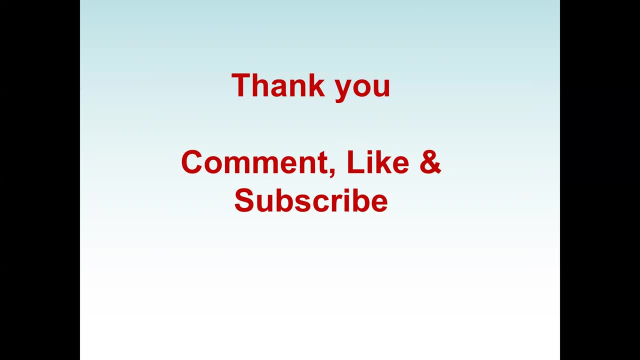 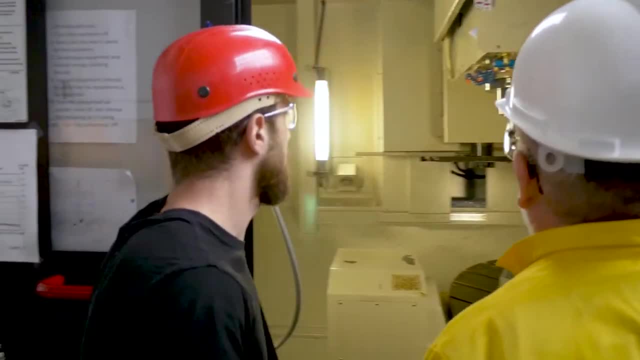 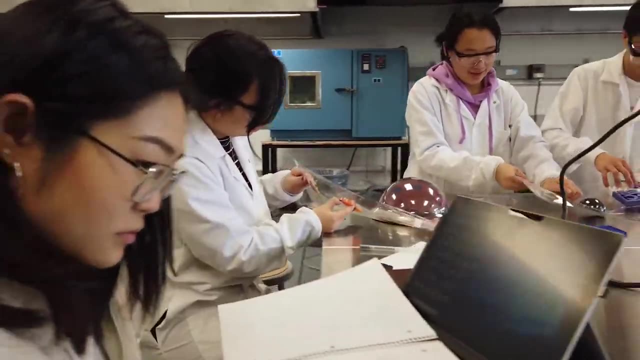 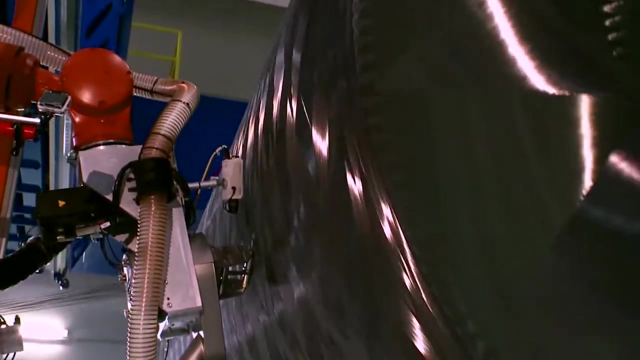 The future of manufacturing is really very different from its past, because this digital disruption will change things dramatically. Everything you use in your daily life must be manufactured. It's important to get education in manufacturing as early as possible, because all of these industries are looking for people with specific skills. A manufacturing engineer. 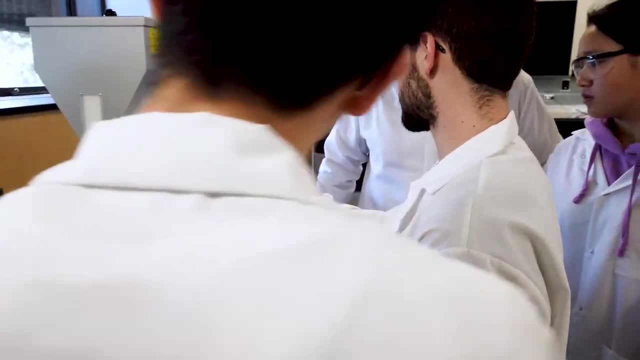 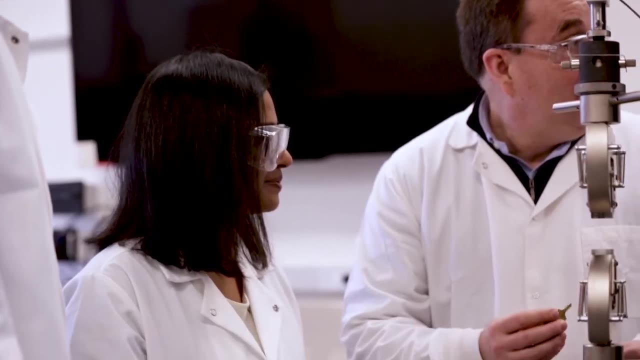 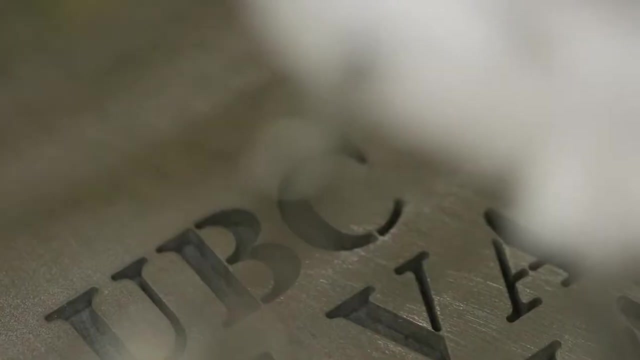 has to be able to do design, engineering, analysis and manufacturing processes. So a specific example for manufacturing in the future might involve something quite different than what we think about today. We've been in discussions with our biomedical engineering program about making blood products and tissue products to optimize and come up with better ways to 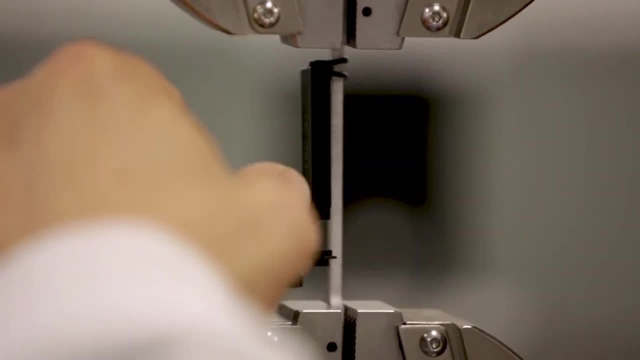 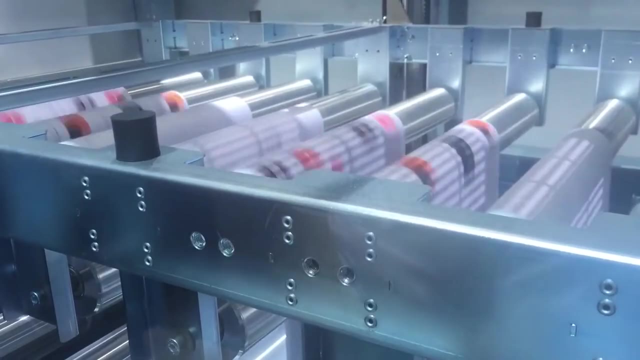 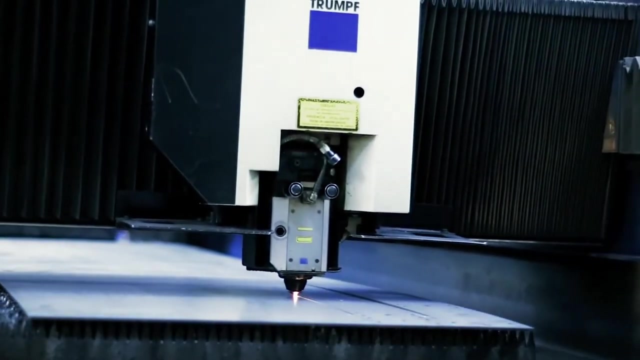 make the products that they need. Manufacturing means that you're producing an idea into a product that you can actually use and interact with. Manufacturing engineers typically design processes. It starts from the raw material to the final inspected part. Manufacturing is really neat because you bring ideas into reality. Lots of engineering disciplines are focused on 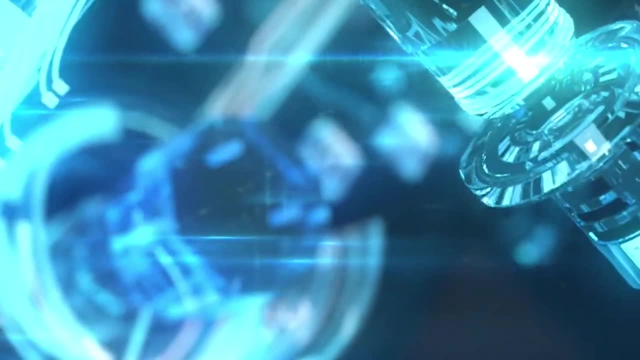 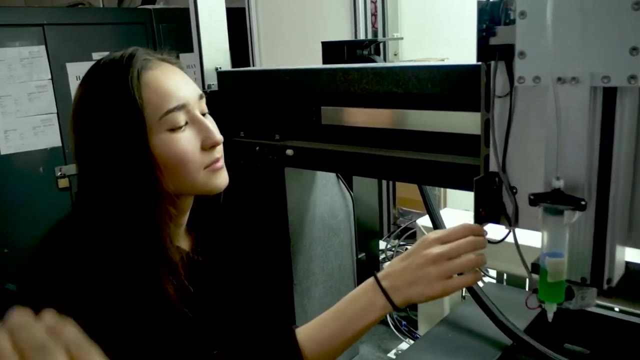 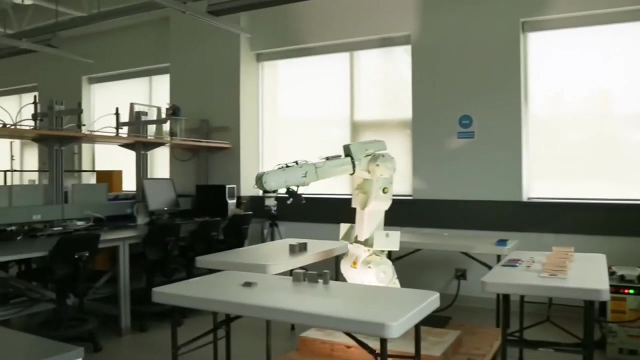 designing them, but manufacturing really brings that design into reality. It appeals to me because I've always been really interested in technology, and that's essentially what manufacturing is. It's heavily mechanical, electrical controls focused, and all of those things are applicable to working on future technologies that are relevant to everybody. 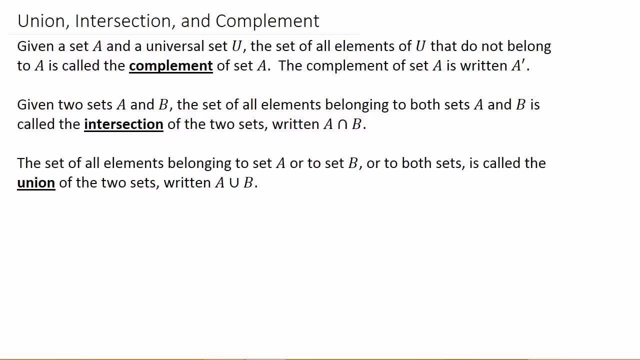 All right. so this video we're going to look at sets and we're going to talk about union, intersection and complement. All right, so let's talk about what each one is. If we're given a set A and a universal set U, the universal set is the set that contains everything. okay, And the set.